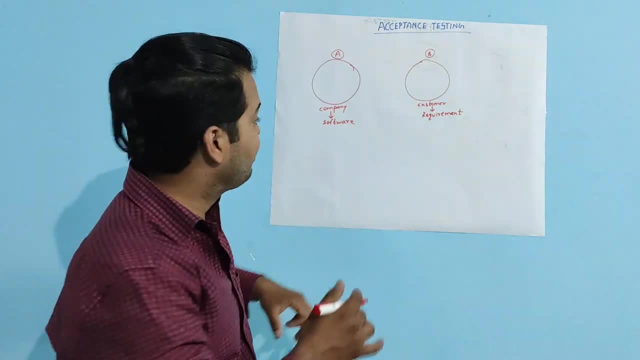 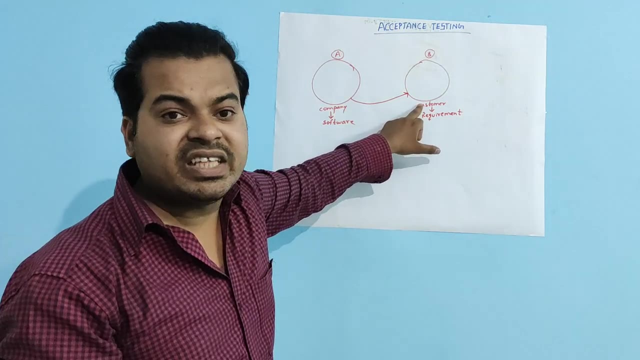 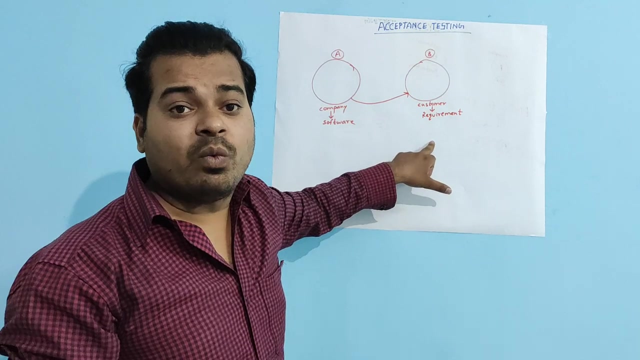 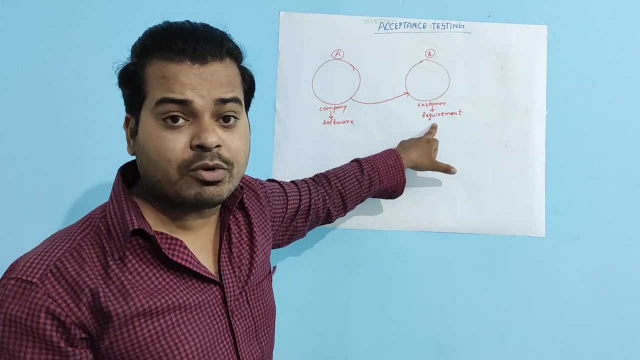 And they will give the software to them. They will build the software and give it to them. How company will decide whether they have to take up the software or not. They will do acceptance testing to make sure that whatever the software this company have developed is according to the requirement they gave at the starting of the project. 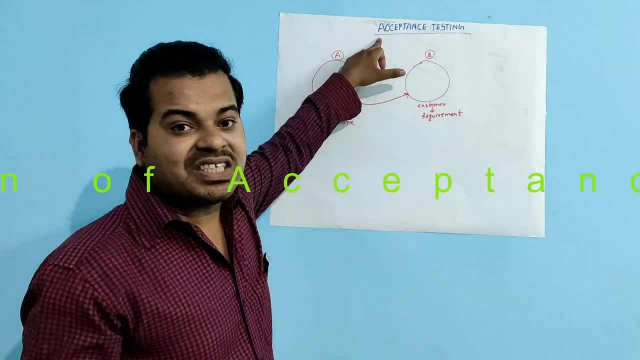 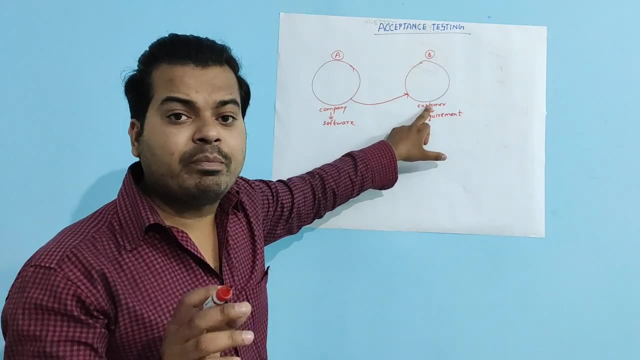 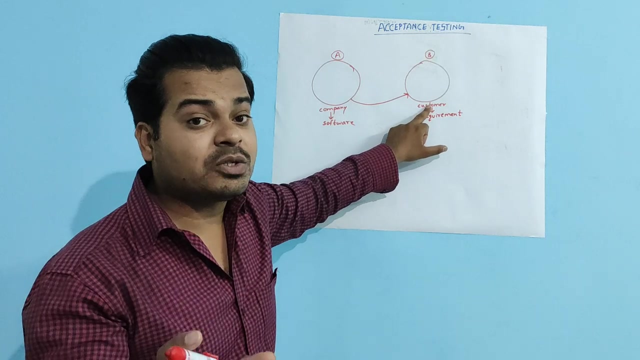 So what do you mean by acceptance testing? Acceptance testing is nothing, but It is an end-to-end testing which is done by my customer for a particular period of time to make sure that software is able to handle real-time business scenarios or not. 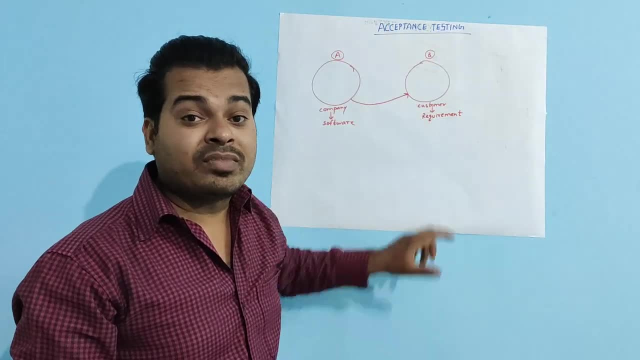 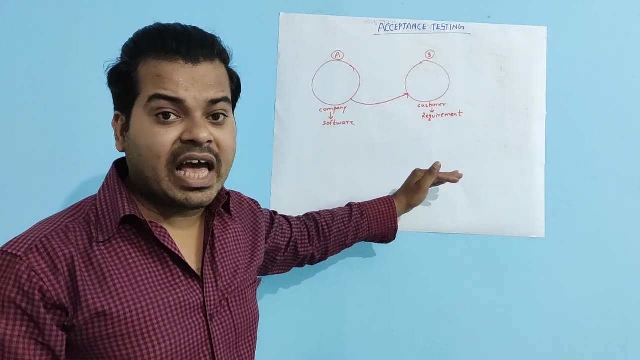 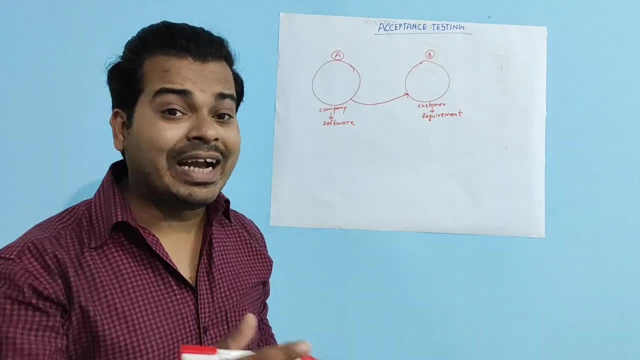 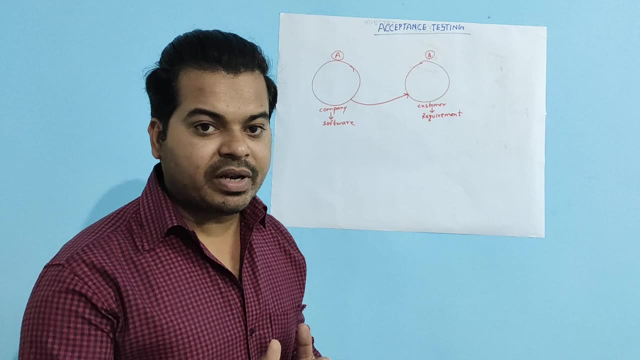 That is called as end-to-end testing. If you guys are making this end-to-end testing, make sure that you watch my system testing video and just come to this video. In some companies, acceptance testing can also be called as UAT- User Acceptance Testing. 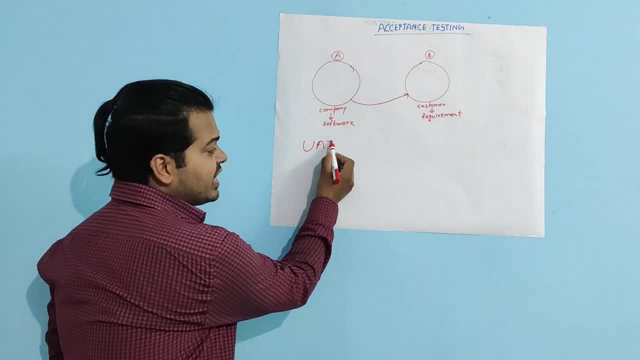 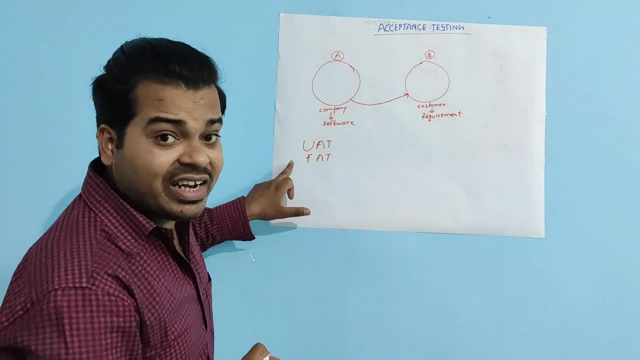 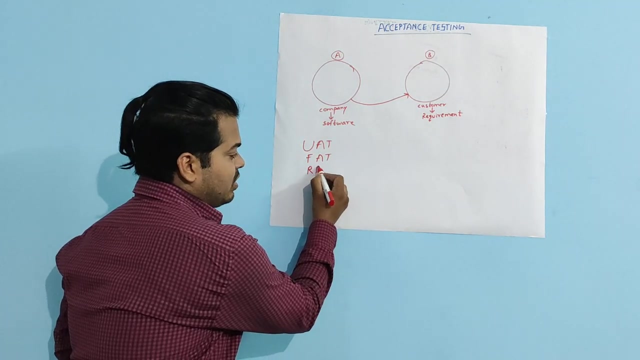 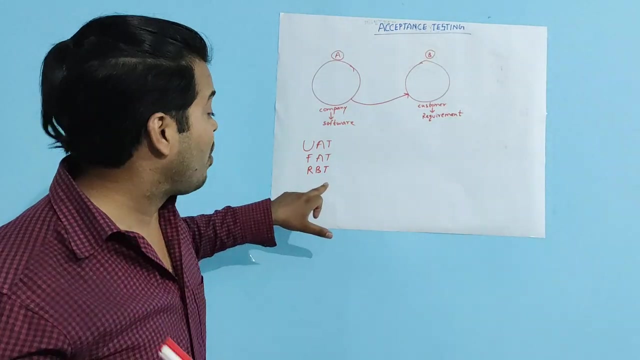 For these include URL and CODE- User acceptance testing. In some companies it is also called as FAP- Final acceptance testing. in some companies it is also called as RBT- red box testing. why it is called as red box testing is because it is the last stage of the testing before giving. 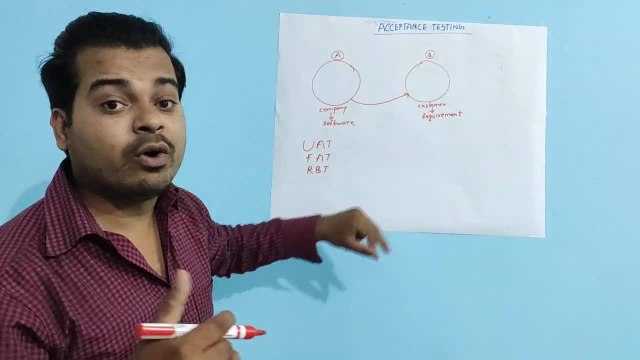 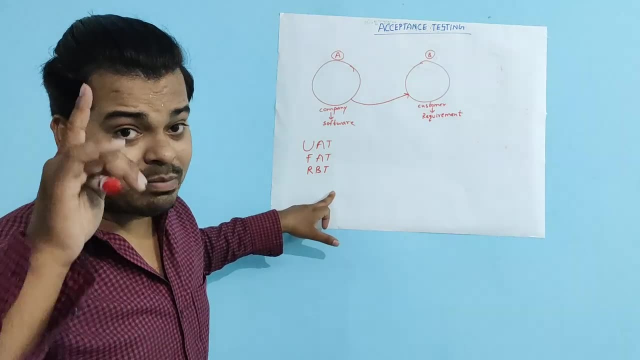 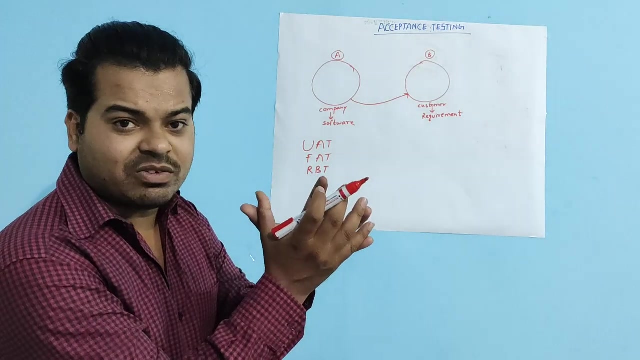 the software to the customer. I hope it is understandable. this can be a tricky question in interview can be asked: what do you mean by RBT? make sure that you remember the reason: RBT, red box testing. why it is red color? because it is the last stage of testing guys. now the question arises in how many ways this 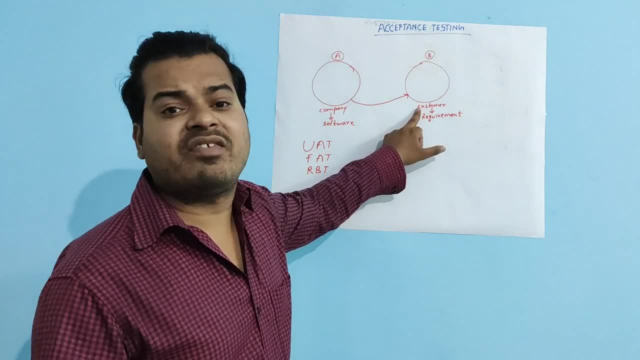 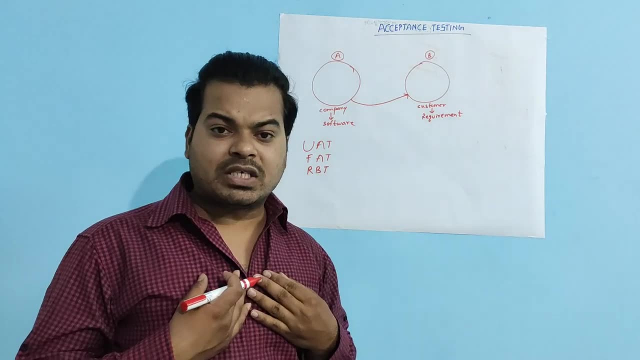 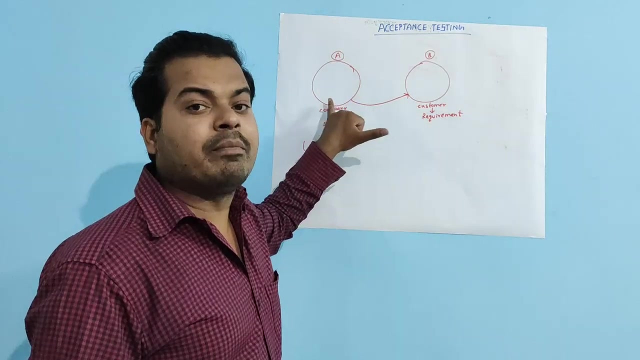 customer can do acceptance testing. the answer varies from person to person. you just think from your point of view. if you are a customer, if I am some customer, I have requested that my software should work like this and I have given a requirement to some company company have. 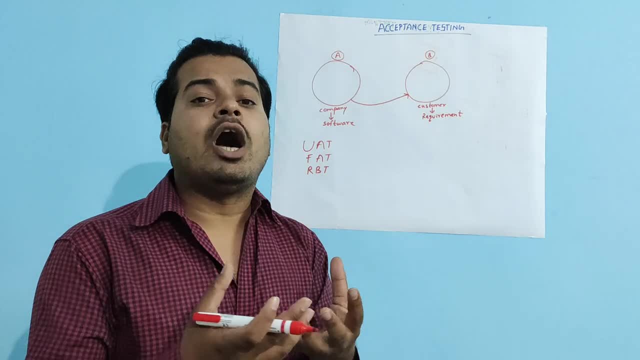 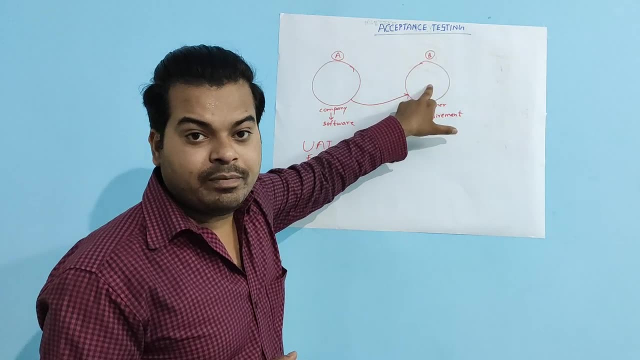 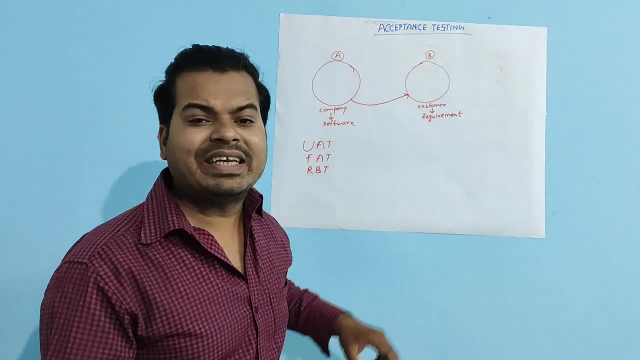 made the software they have given it to me. now in how many ways i can do acceptance testing. you just think about it. so there will be people who will be working in my company. right, i will, let's talk about it. engineers will be working in my company, or a agent will be working, or my any. 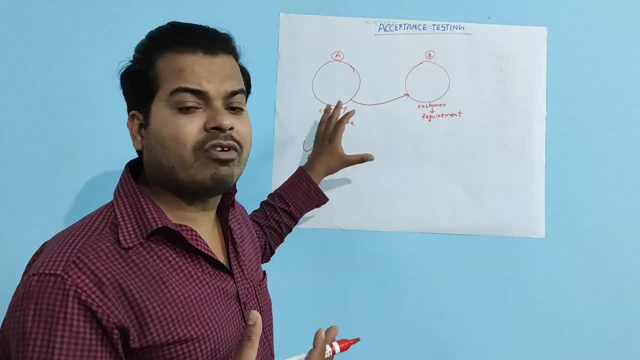 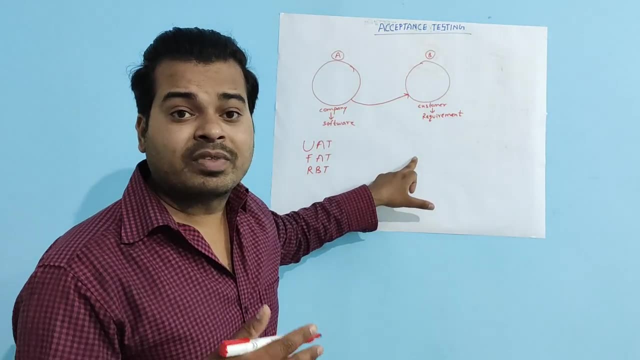 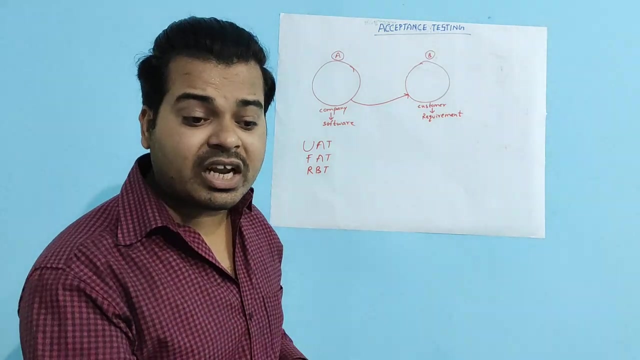 technical team who is aware what requirement we have given to the, to the customer, so those people can perform the testing on that software which is given by the company by real-time business scenarios. they won't look into the requirement and test it. they will do the testing by using it. 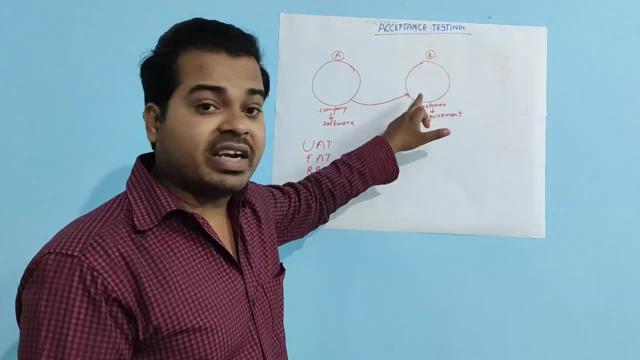 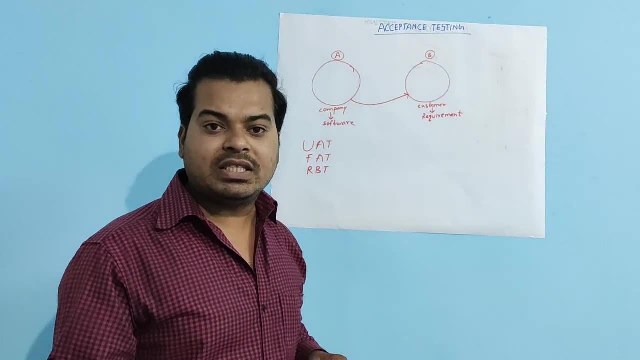 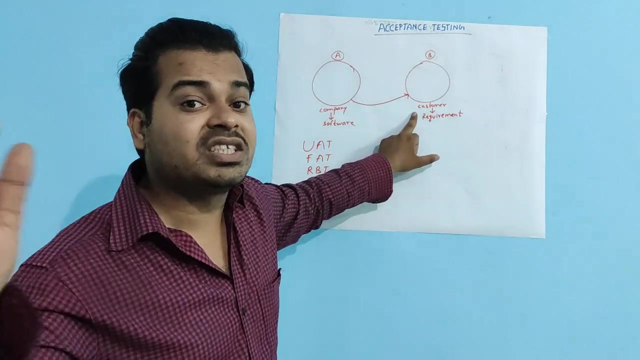 in real-time. real-time business scenarios. they are going to test it and make sure that software is working as expected. when i say real-time business scenario is it means how customer is going to use a software to run their business. that is called as real-time business scenarios. guys, when this company made the software and 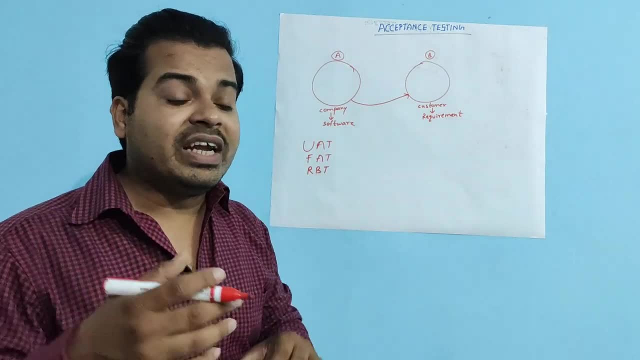 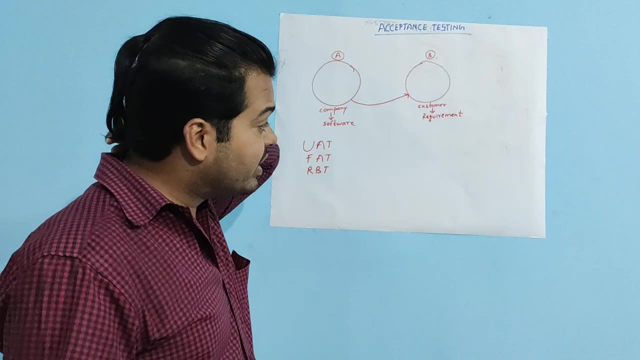 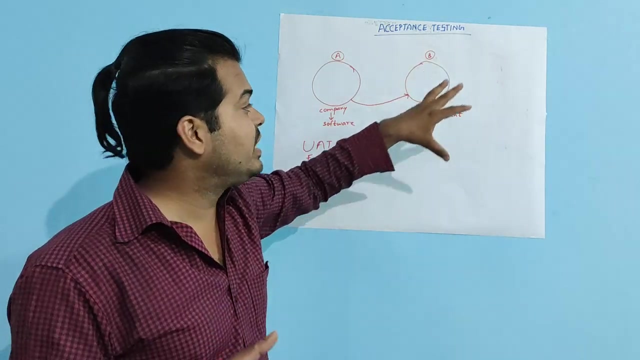 qa tested it. they didn't tested it by entering the real-time business scenarios. they entered some dummy values and they tested it here. but when it comes to the acceptance testing and this, this customer's it engineers or agent or any technical team present in this company- when they are doing acceptance testing, they will enter. 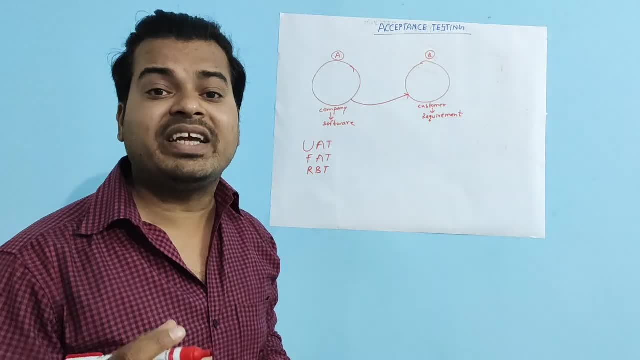 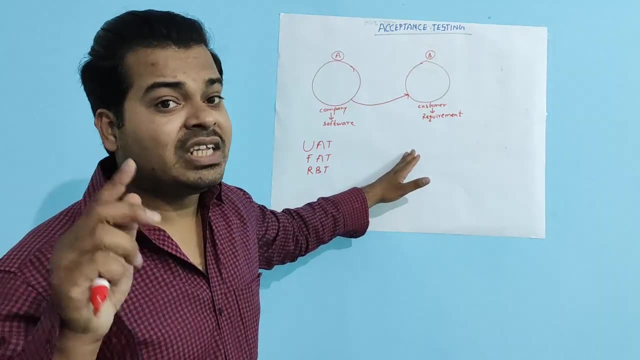 you, they're going to test. they're going to test the software by entering real-time business scenarios and they're going to test it whether it is working perfectly fine or not. make sure that they are not going to test the software by looking into the requirement. they're going to test the 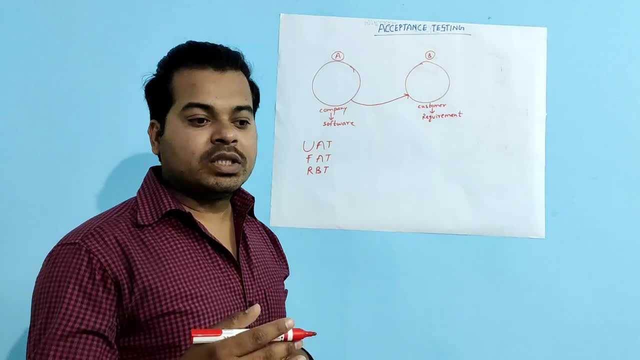 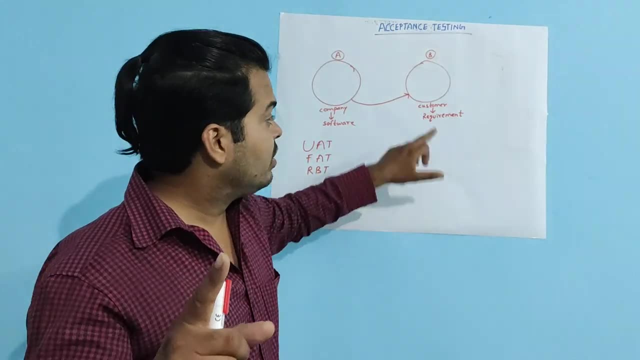 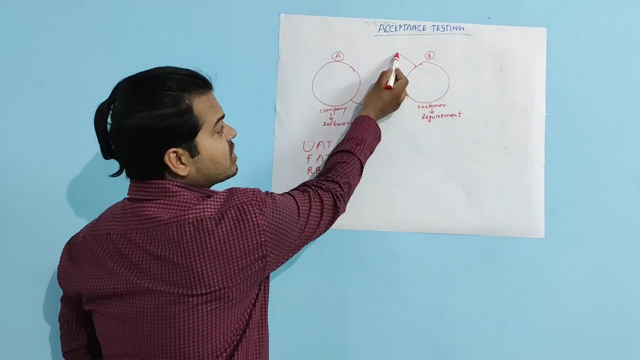 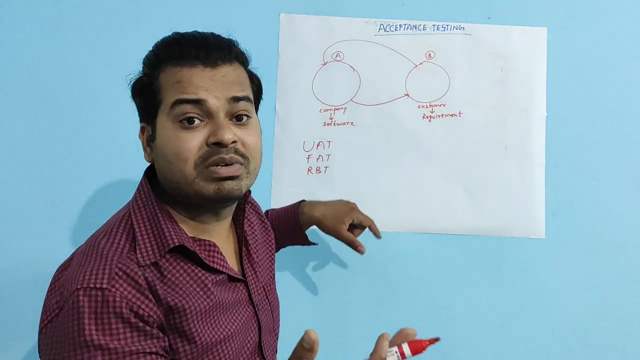 software by entering real-time business scenarios. the another way by which customer can do acceptance testing is one person from this customer place, let's say one it engineer- will fly to this company place, or else he will go to this company place with set of real-time business scenarios, with a set of real-time business scenarios in a sheet, and 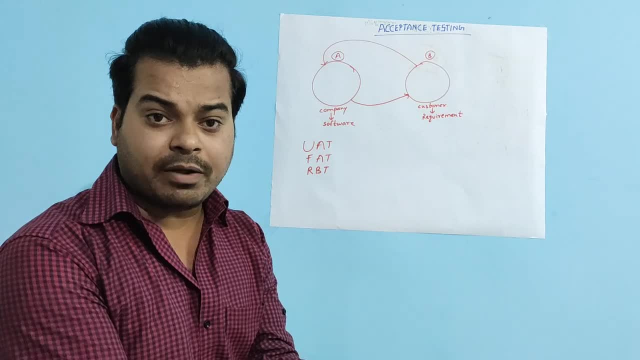 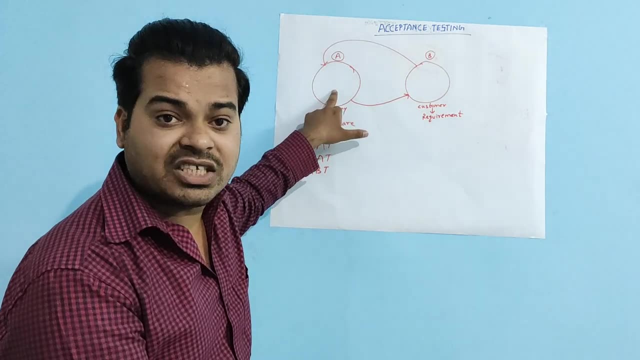 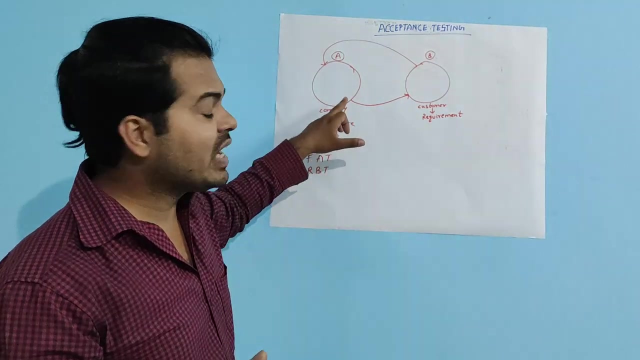 he will give those sheet to the test engineers present in the company and he gonna tell them that perform all the scenarios and test my application. this is one more way of the accepting acceptance testing. There is one more way by which we can do acceptance testing is by making a test engineer of this. 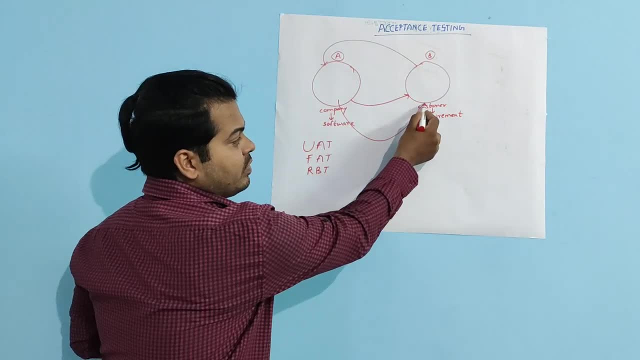 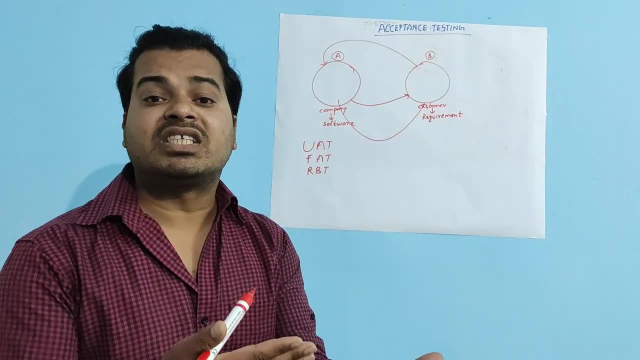 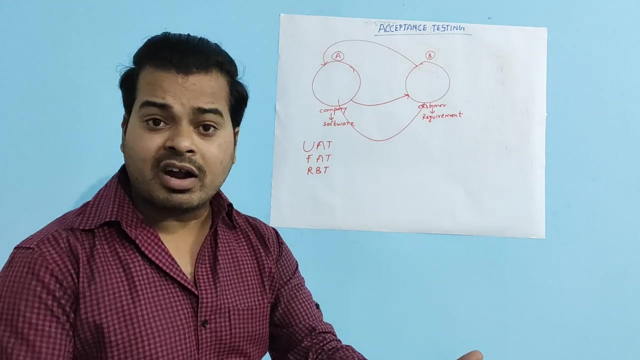 company fly to this company. That means test engineer present in this company will go to the customer place and customer will give him the real time business scenarios that these are the scenarios that you need to perform on the application and make sure that it is working perfectly fine or not. 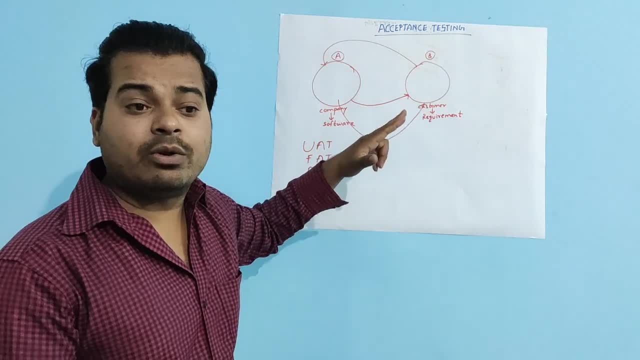 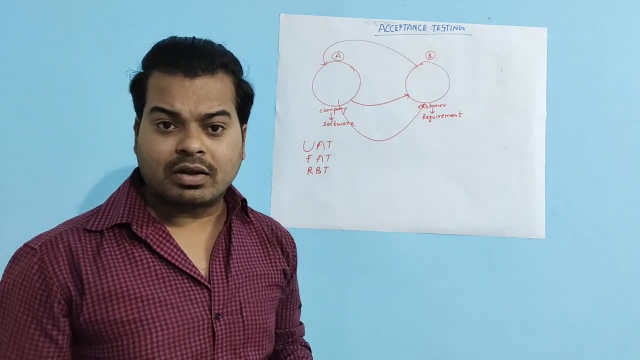 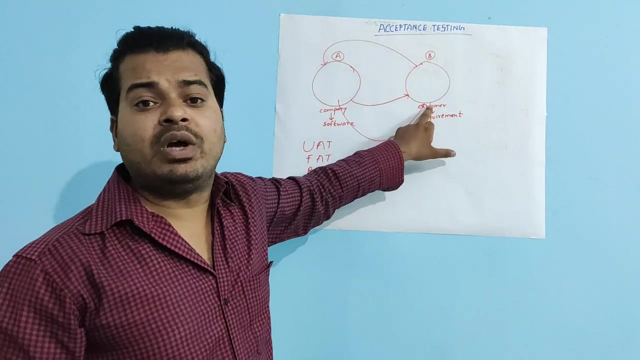 So test engineer will use the software by looking into the scenarios. my customer wants me to do it and then they will make sure that the software is working perfectly fine or not. This is how they are going to do the testing. One more way by which customer can do acceptance testing is they will release the software. 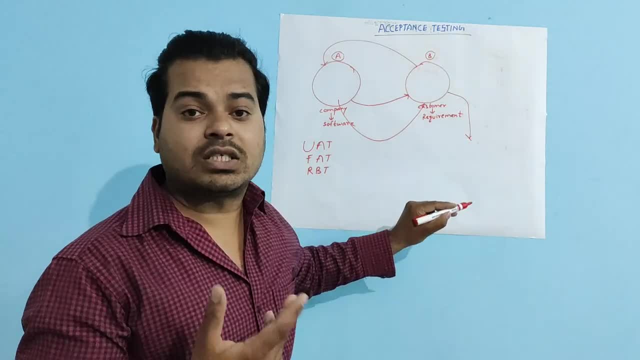 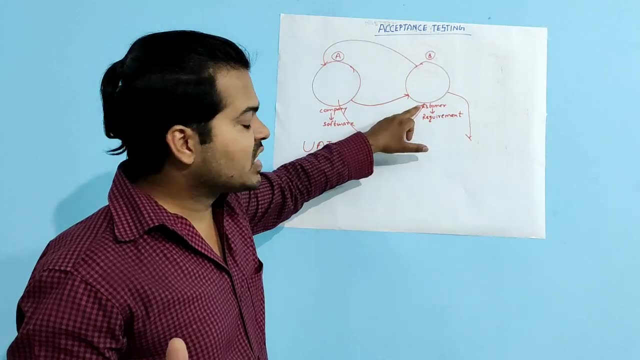 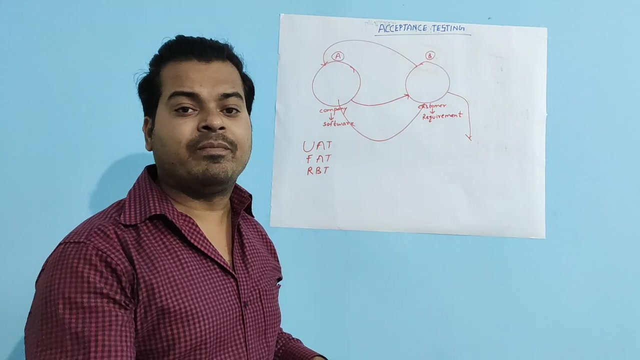 to the customer. They will release the software to their customer. Let's say, this customer is there, right? they want to release the software to their customer and ask the customer to use it and test the software whether it is able to handle our business scenarios or not. 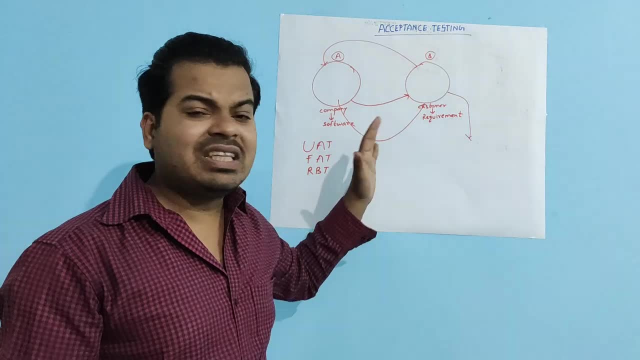 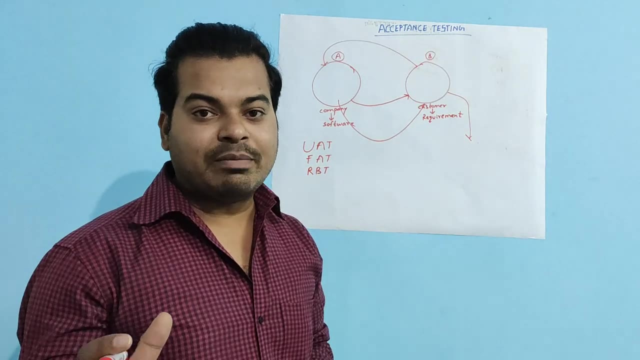 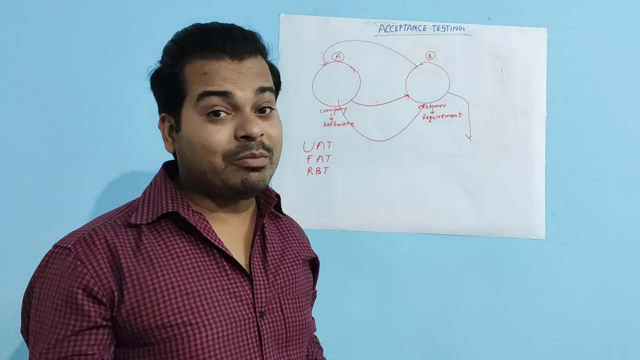 So their customer will only test their software. So these are the various ways by which customer usually do acceptance testing. I hope I was able to make you guys understand what do you mean by acceptance testing. if yes, please share. Like this video, subscribe to my channel and please share this video with your needy friends. 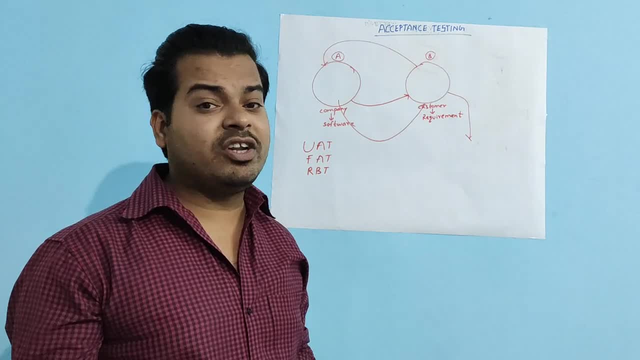 who are looking for a job. Please hit the bell icon to never miss any video from software testing by mkt in future.